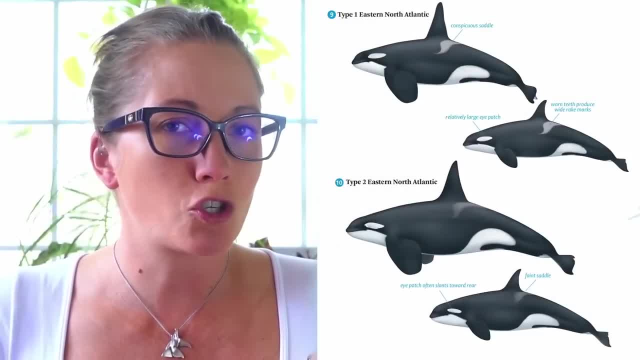 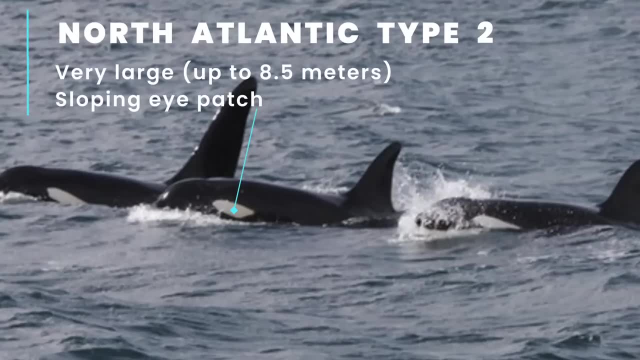 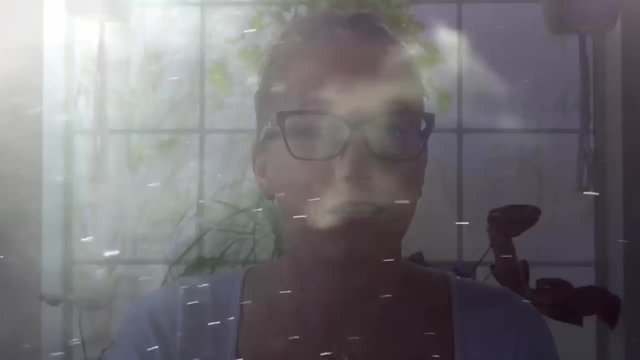 appearance and hunting behavior. For example, there are two recognized ecotypes in the North Atlantic. Type 2 orcas are very large with a sloping eye patch and they prey on small baleen whales like minke whales. Type 1 orcas are much smaller than type 2s. They primarily 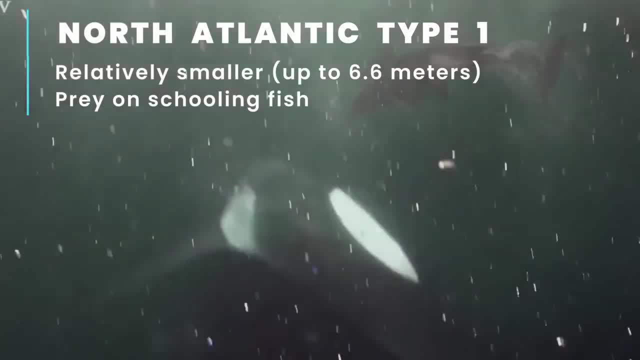 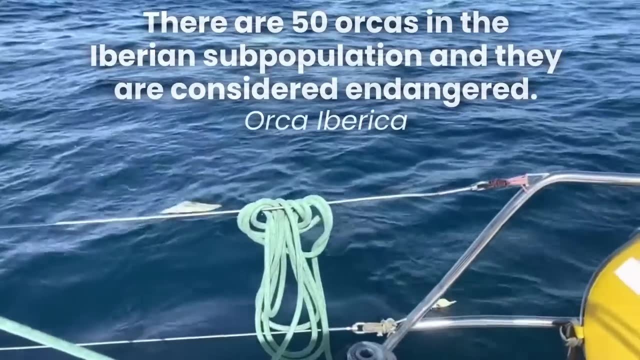 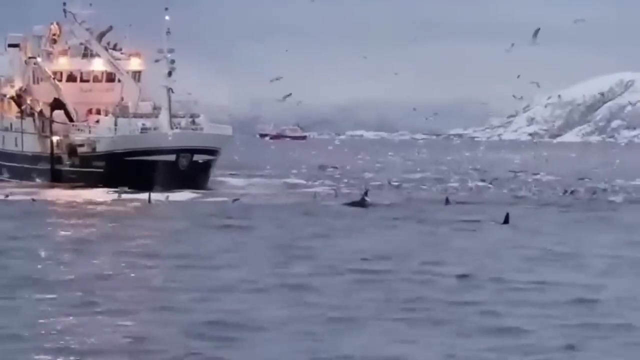 feed on herring, mackerel and tuna that they cooperatively herd into dense schools. But within these ecotypes are distinct breeding populations. One of these Type 1 populations is the Gladys orcas. Another Type 1 population lives off of the coast of Norway and has 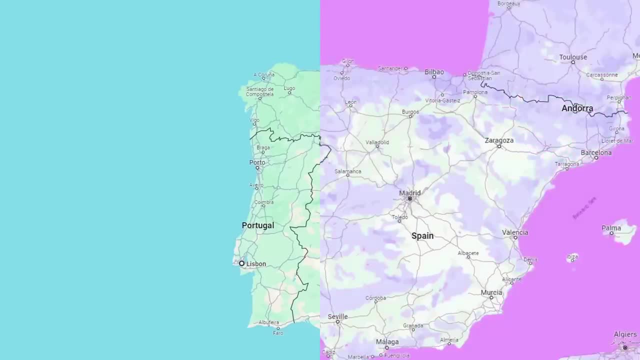 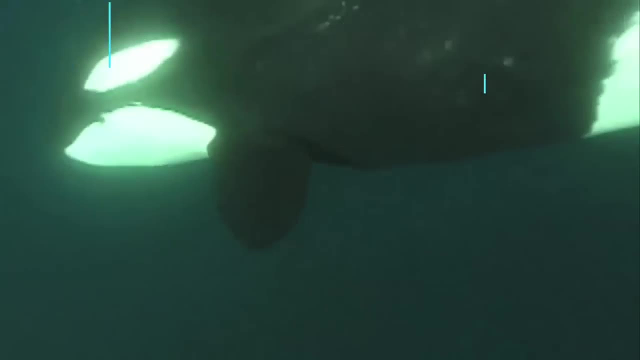 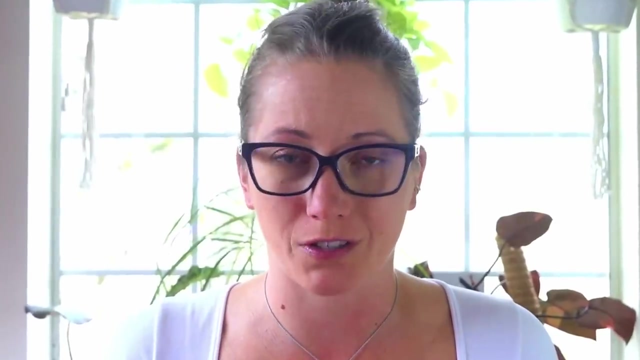 learned how to steal mackerel out of fishing nets. These two populations live thousands of miles away from each other. They do not interact at all and have their own language, language, social structure, food preference, hunting behavior- essentially their own culture. 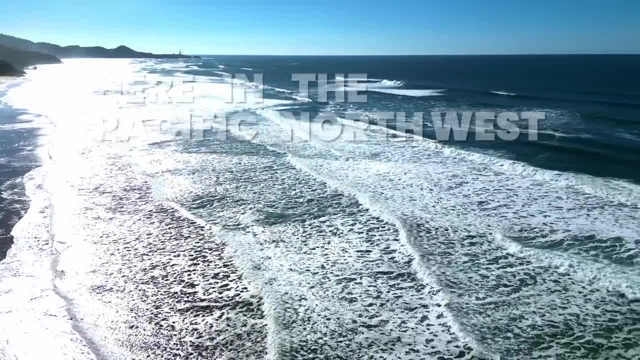 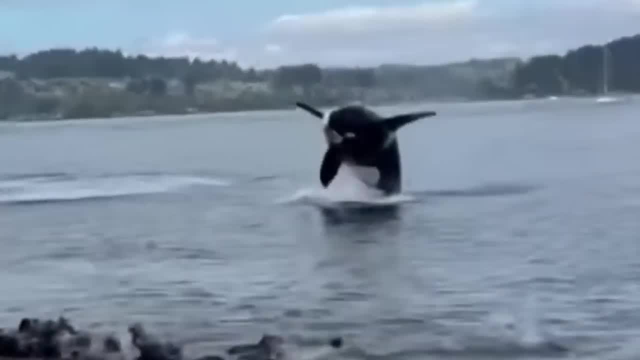 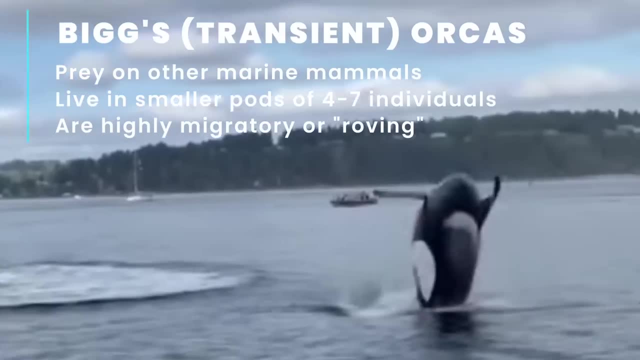 for lack of a better word. Here in the Pacific Northwest we have the resident bigs and offshore ecotypes. Bigs, also known as transient orcas, prey on other marine mammals like seals and sea lions. They live in small pods, usually around five individuals, and most of these pods are extremely 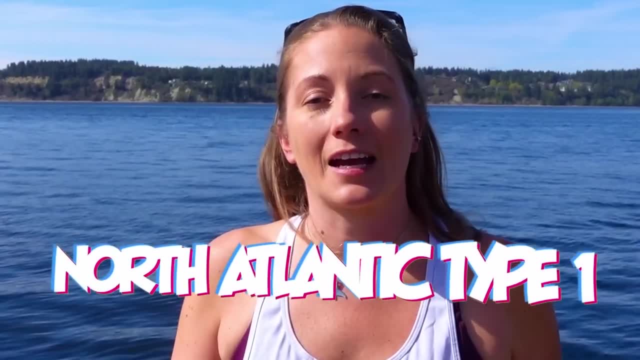 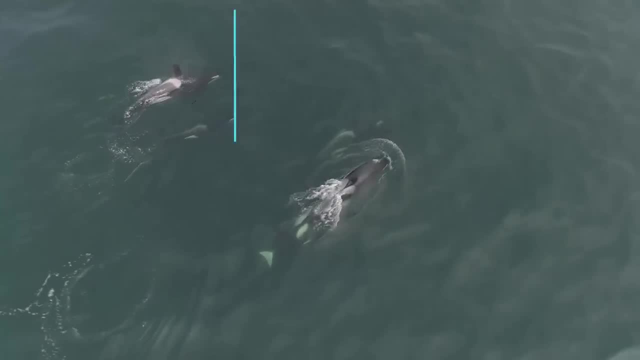 migratory Transient orcas are similar to the North Atlantic type 1 orcas. They're smaller, live in larger pods and are relatively docile salmon eaters. The offshore orcas, as their name suggests, live offshore near the continental shelf. 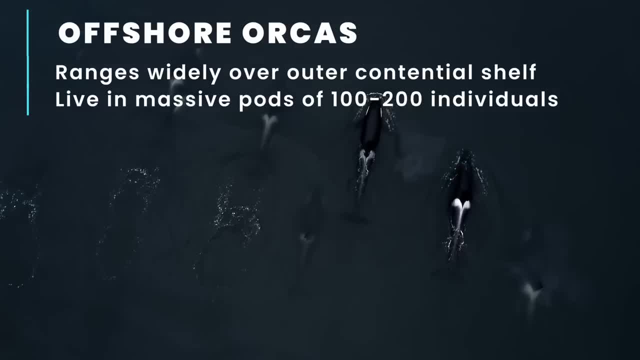 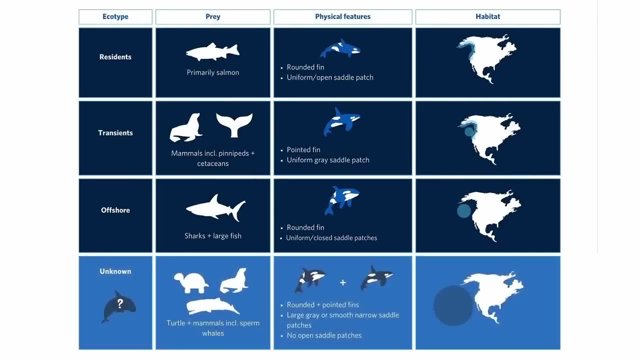 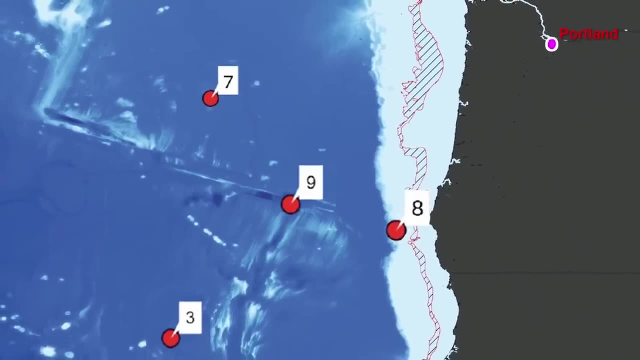 in massive pods that can number in the hundreds. They almost exclusively eat shark livers. Now researchers have potentially discovered a fourth ecotype that lives even further out into the open ocean, Hundreds of miles beyond even the continental shelf. A clue to the new population's presumed habitat lies in the cookie-cutter shark bites that. 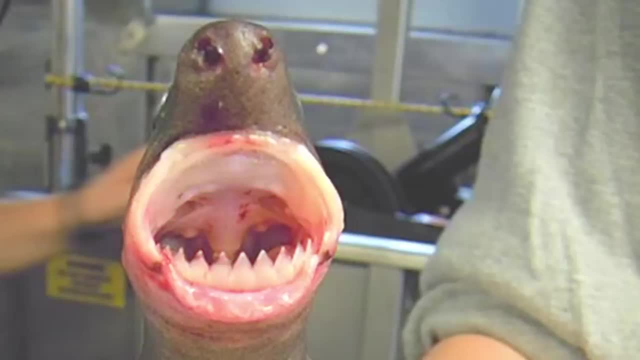 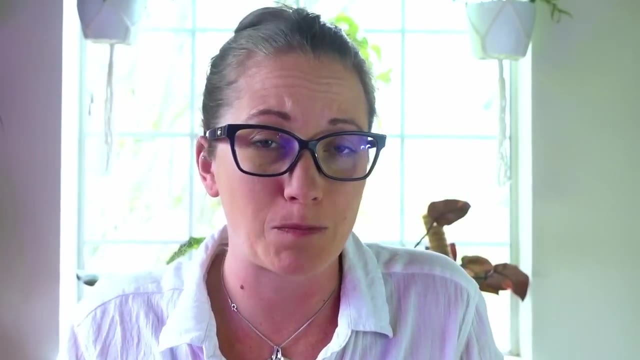 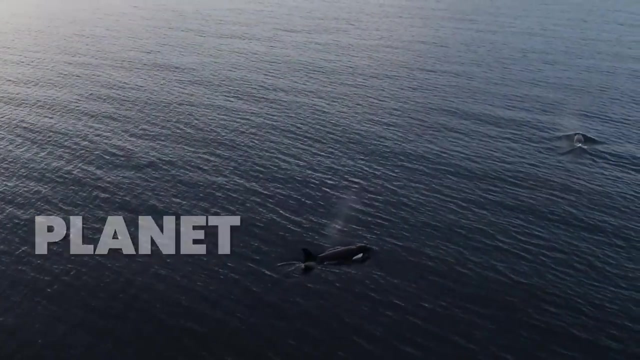 are seen on almost all of the orcas in this pod. These parasitic sharks live in deep waters far offshore. This remoteness makes gathering information on this population quite the challenge. The open ocean is the largest habitat on our planet and observations of killer whales. 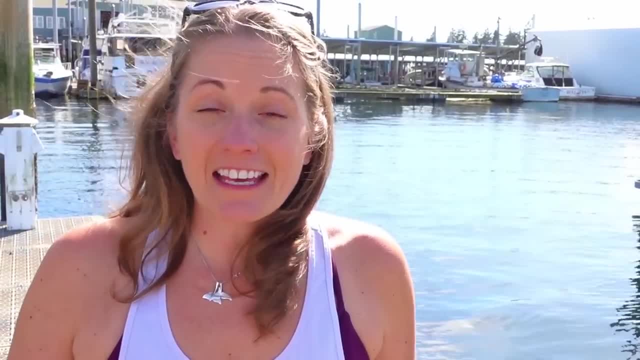 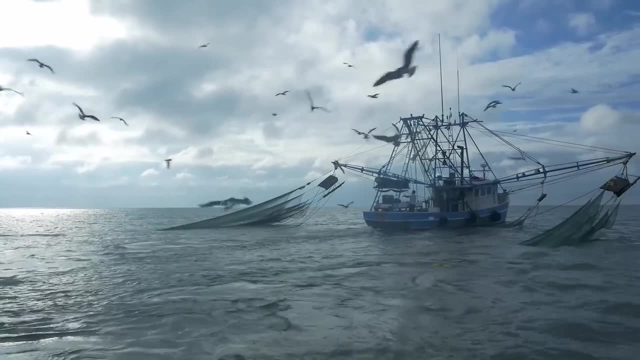 in the high seas are rare, But, according to research, the ocean is the largest habitat on our planet And, according to researchers, they're actually getting help from some local fishermen who are taking cameras in order to get video of these specific orcas and their encounters. 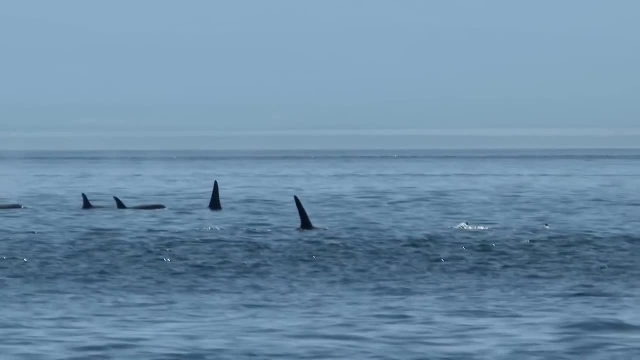 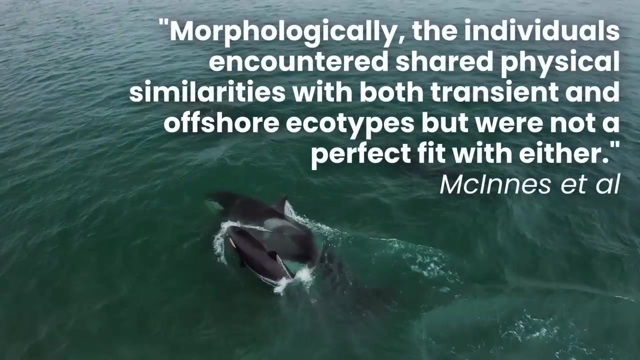 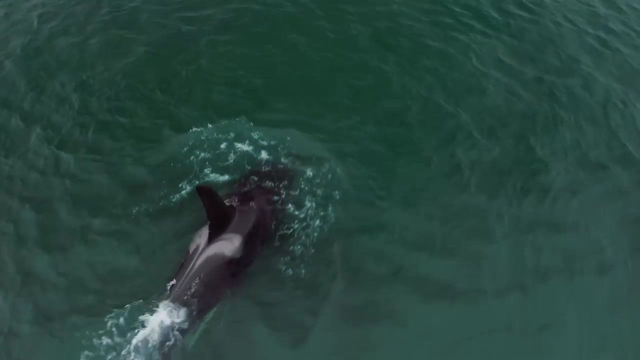 with them. The 49 killer whales could not be matched with any known animals through photos or descriptions. Morphologically, the individuals encountered shared physical similarities with both transient and offshore ecotypes, but were not a perfect fit for either. But it's this population's aggressive hunting behavior that has shocked researchers. 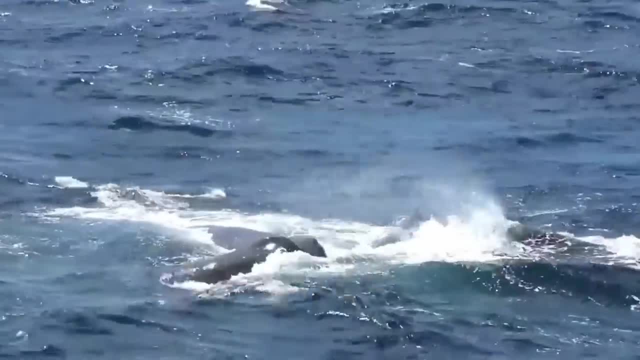 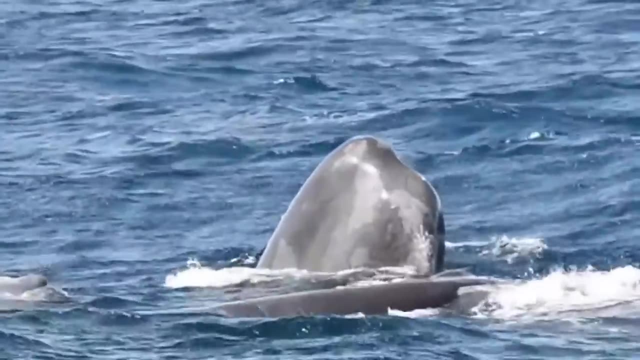 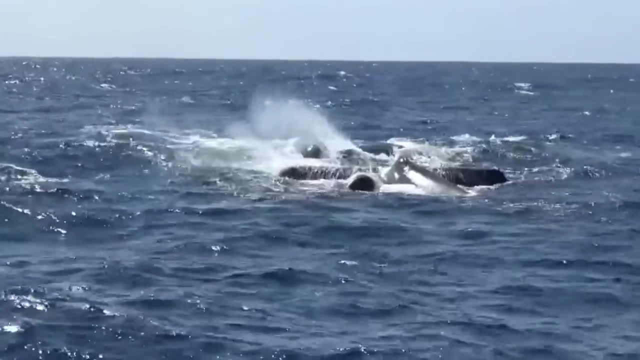 So let's take a look. In one of the first encounters researchers had with a pod of these oceanic killer whales, they were observed taking on a herd of nine female sperm whales: Nine, Nine, Nine, Nine, Eventually making off with one. 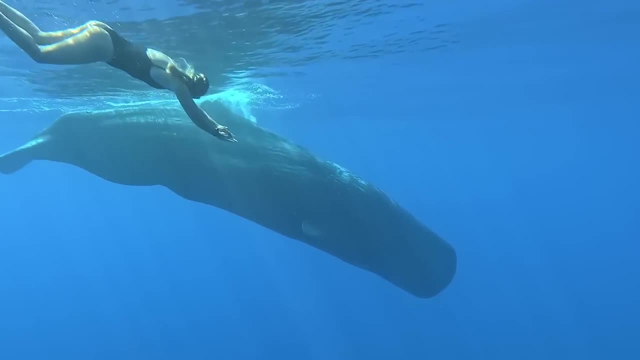 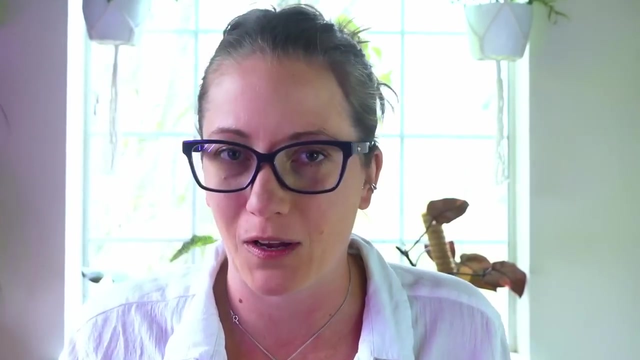 This is wild. Sperm whales are the largest of the toothed whales and the largest toothed predator on the planet currently, And this is the first time killer whales have been reported to a zoo. This is the first time killer whales have been reported to a zoo. 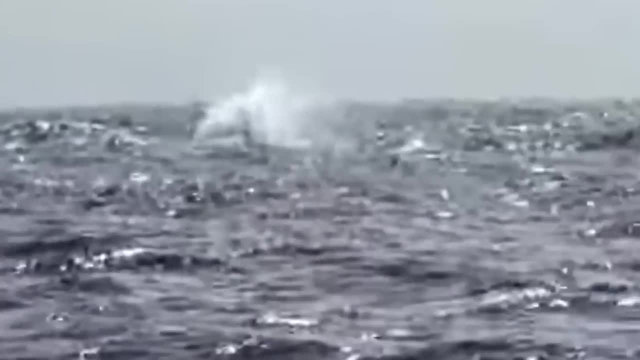 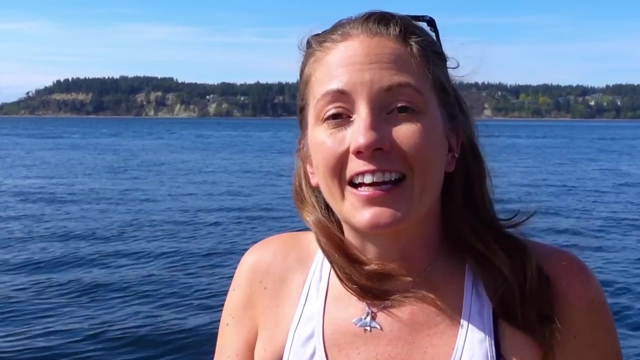 This is the first time killer whales have been reported to attack sperm whales on the west coast. Other encounters included an attack on pygmy sperm whales and northern elephant seals. Next steps for the researchers is to actually collect DNA samples from these orcas to figure. 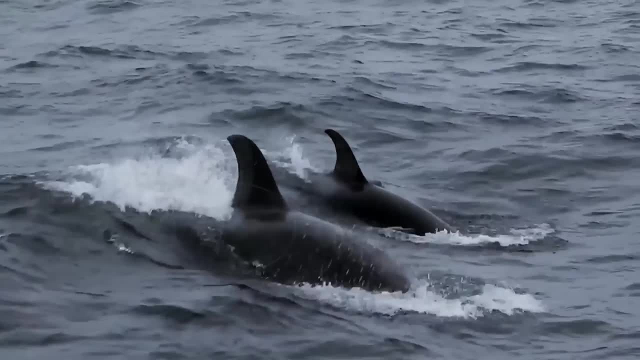 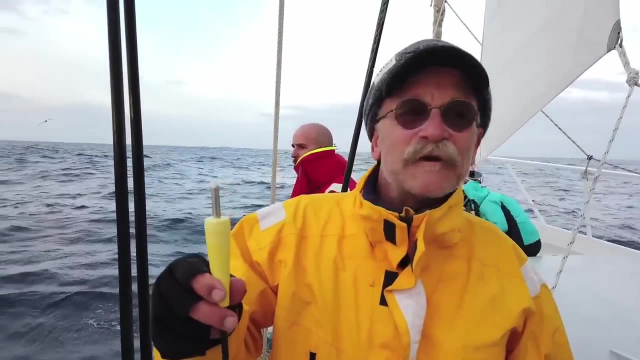 out exactly how far removed they are from other ecotypes. We've got the first ever sample of a type B killer whale- maybe the answer to our questions right here. That's where the second study that I mentioned comes into play. While it might not be as 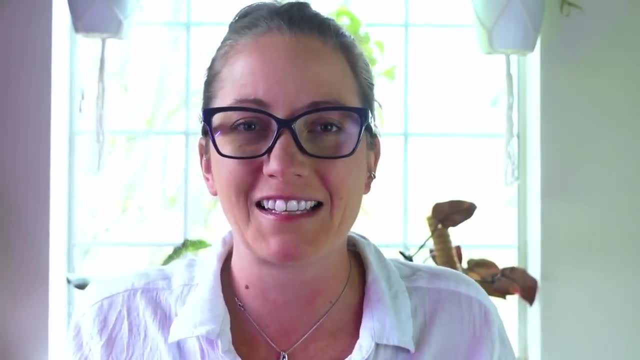 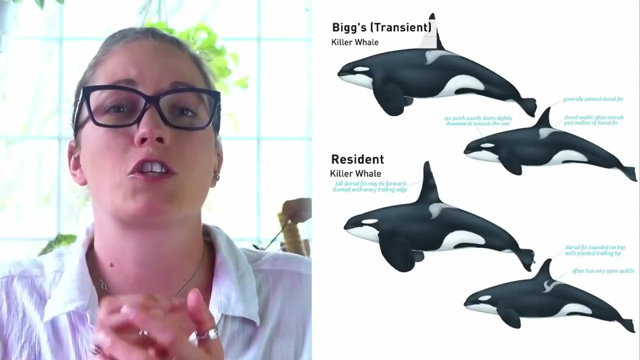 dramatic as a new population, it's still a very interesting study. It's a study that's going to be very popular. In a population of hyper aggressive killer whales taking on sperm whales and elephant seals, it might be even more important. Earlier I talked about the differences between bigs and resident killer whales. 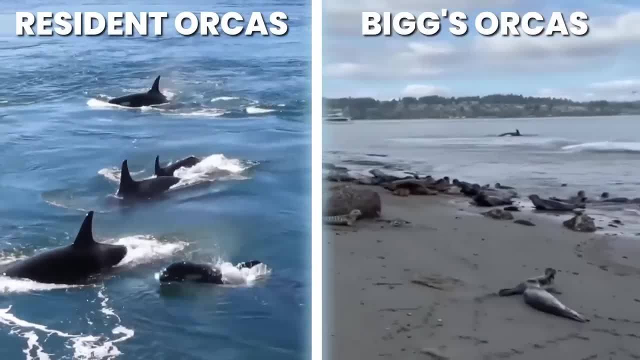 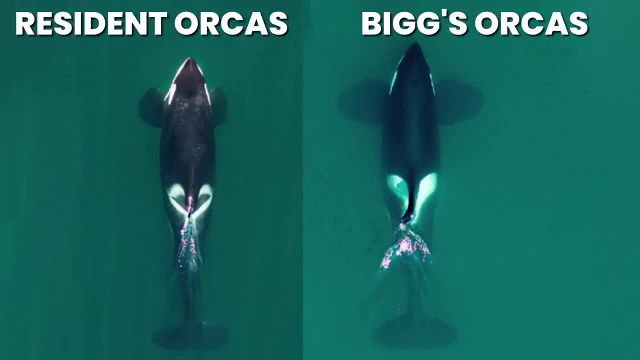 These two types of orca behave differently, eat differently, and they don't even socialize between groups, even if they are in close proximity to one another. They also have several morphological differences. Bigs are generally longer and more robust. The shape of their fins is different and so is the coloration of their saddle patches. 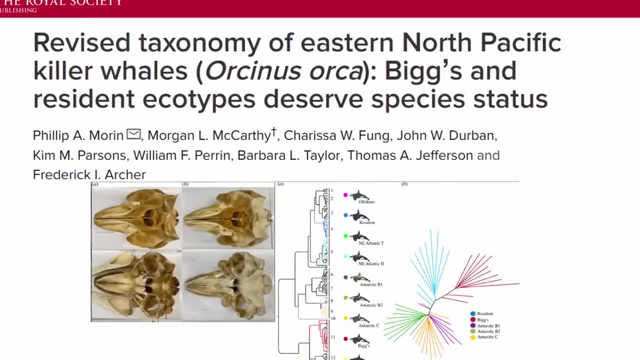 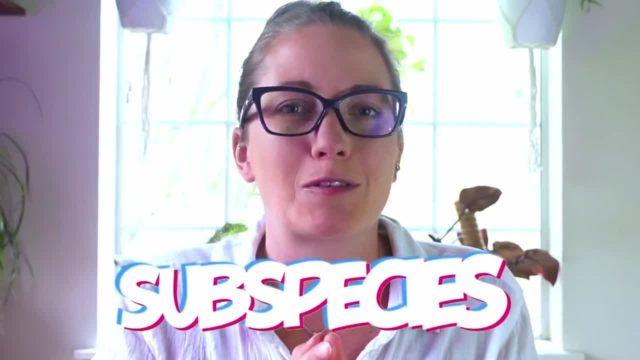 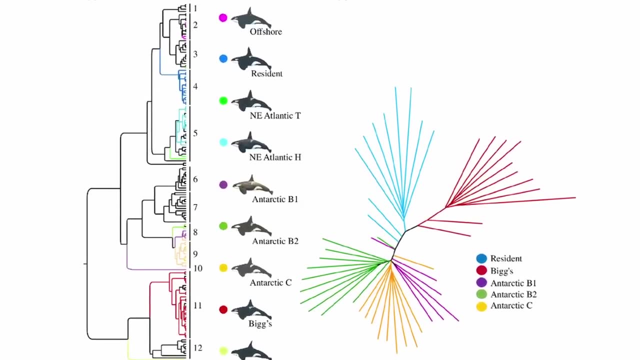 structure is different Now. genetic data from a study published just this week confirms that the groups are not just unique populations, ecotypes or even subspecies, but entirely different species. Genetic analysis found no evidence of interbreeding between the bigs and residents, and that they 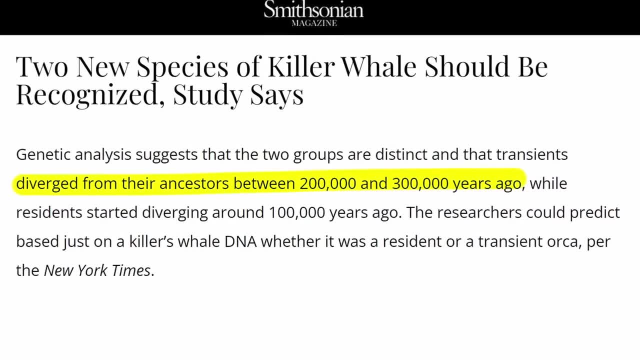 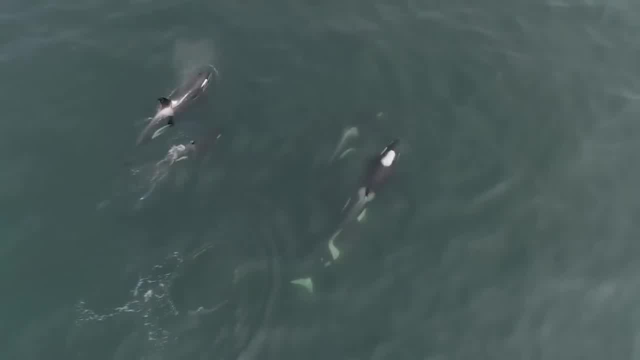 likely diverged between 200,000 and 300,000 years ago. The Society for Marine Mammalogy is reviewing the proposed names for these newly classified species: Orchinus Ader for the resident orcas and Orchinus Receptipinus for bigs. 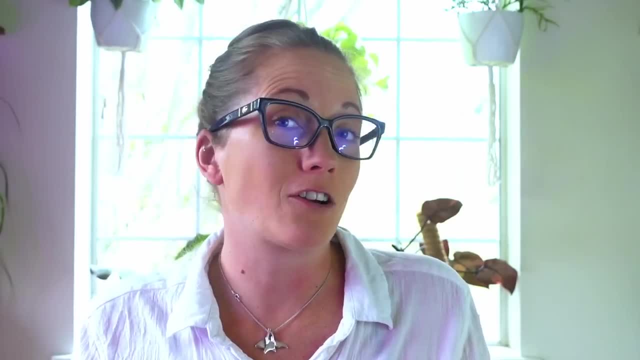 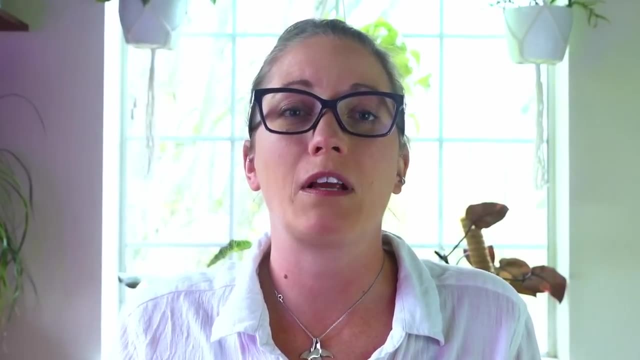 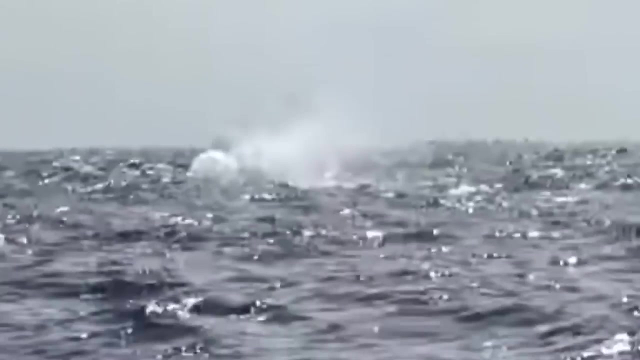 Is it Adder or Ader? Adder, Ader Orchinus, Ader Orchinus. Adder To-mater To-my. This study also lays the groundwork for reclassifying the other ecotypes of killer whales, including the Gladys orca in Iberia, and this aggressive new population that hunts sperm whales. 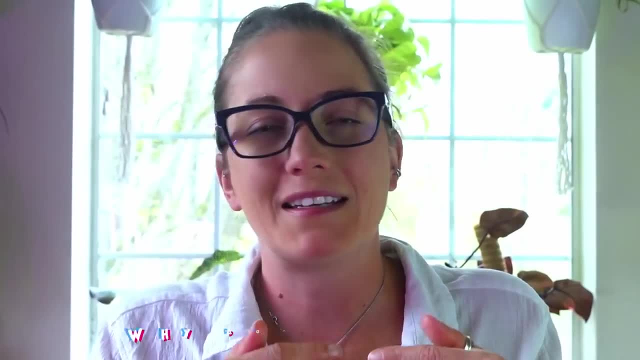 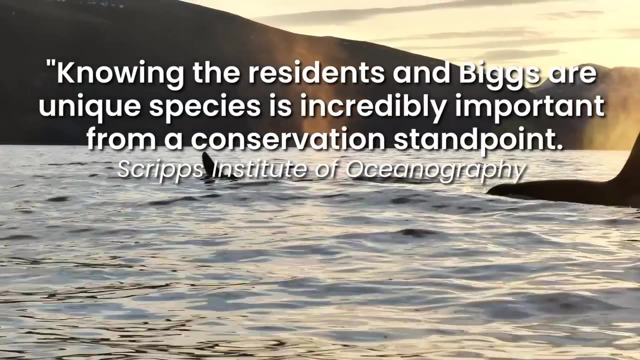 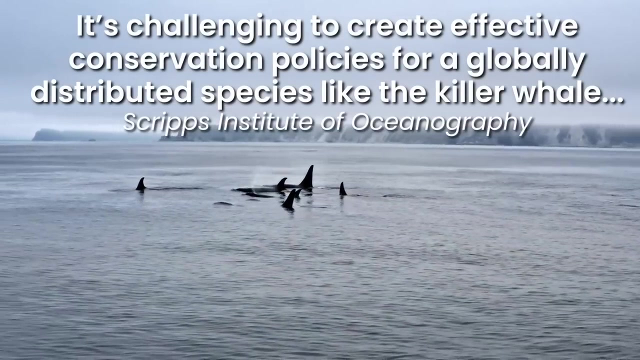 Now why is this a big deal? Why does any of this matter at all? According to the Scripps Institution of Oceanography, knowing that residents and bigs are unique species is incredibly important from a conservation standpoint. It's challenging to create effective conservation policies for a globally distributed species. 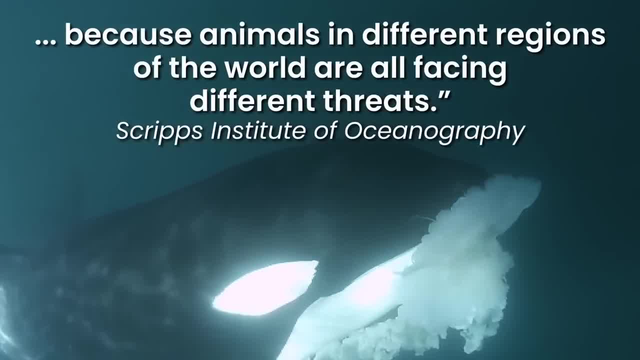 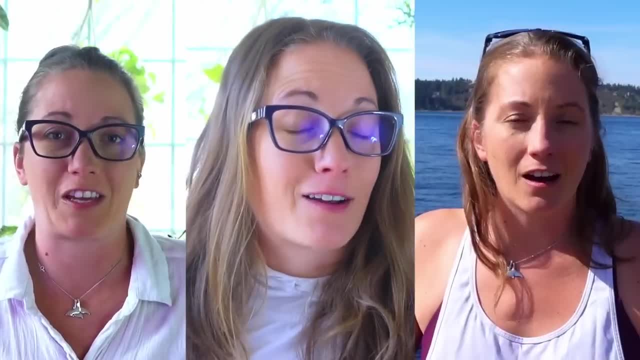 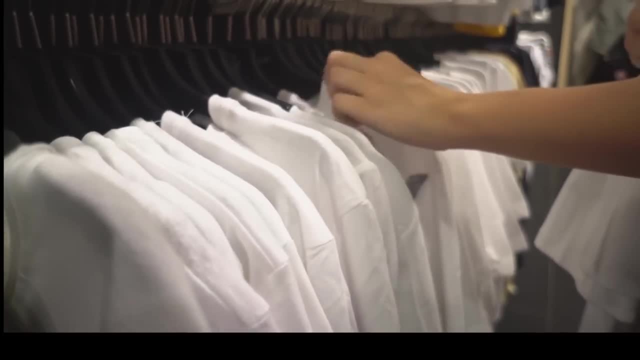 like the killer whale, because animals in different regions of the world are all facing different threats. Think of these different orcas, like my different shirts. Maybe you noticed that I've worn several white shirts in the making of this video. While they all look similar, they're all different styles, brands and even made out. 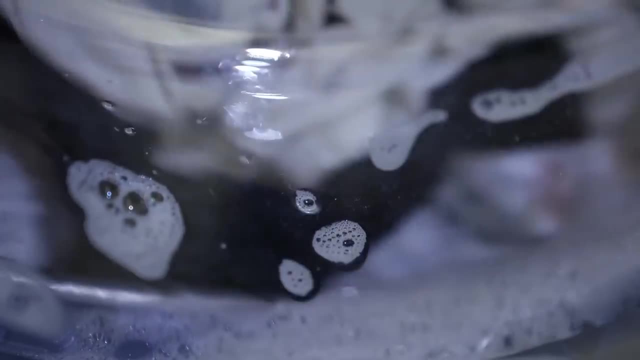 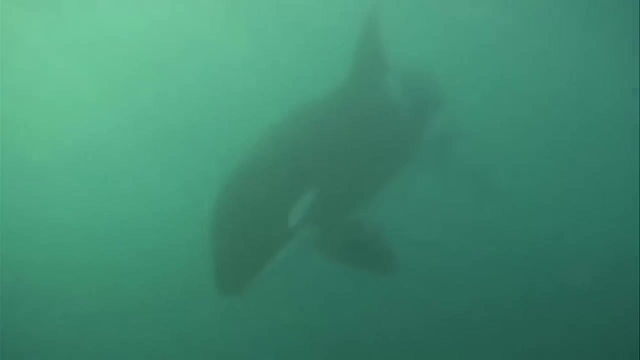 of different fabrics, which means they all need different care. If I treated them all the same, some would do fine, but others would wear out pretty quickly. The same is true for these different types of orcas. For the southern residents, the greatest threat is the lack of food, specifically Chinook. 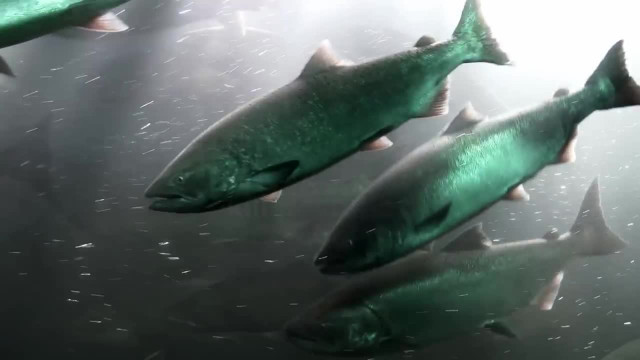 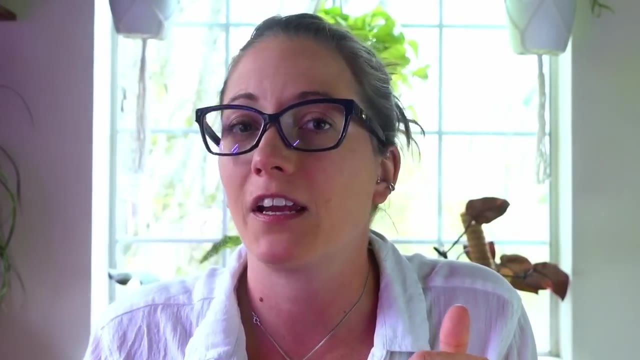 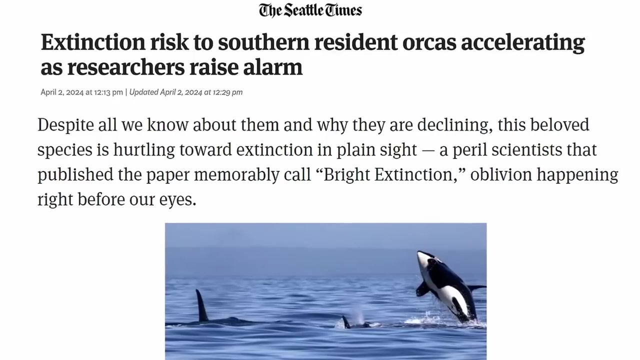 salmon from the Columbia and Snake River systems. This salmon makes up 80% of their diet. This salmon makes up 80% of their diet. A new study that came out literally as we were filming this video and had to re-film this whole portion of it, has shown that the southern resident killer whales are hurtling. at breakneck speed towards extinction. It is expected that within one or two generations they will be gone from the planet forever. Research clearly shows that the survival and reproductive success of these whales is correlated with Chinook salmon abundance. The survival and reproductive success of these whales is correlated with Chinook salmon abundance. The survival and reproductive success of these whales is correlated with Chinook salmon abundance. This is an integral component of the Species Recovery Plan. This is an integral component of the Species Recovery Plan. So how do we increase the population of Chinook salmon? By removing these four dams along the Snake River. 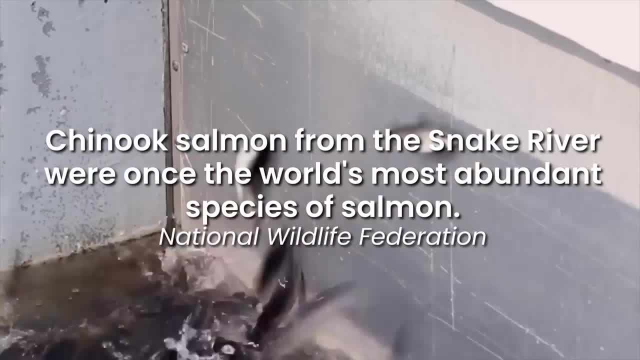 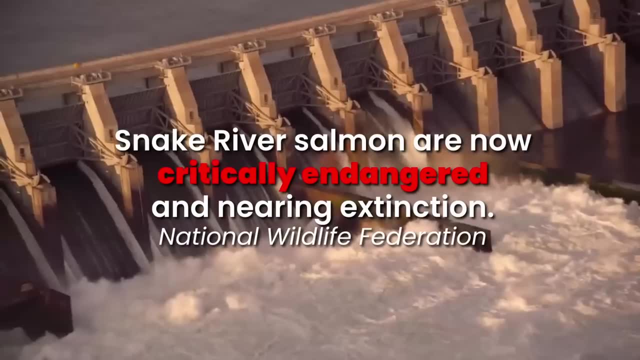 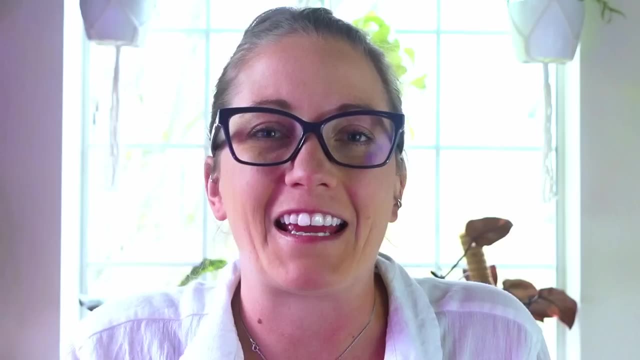 These dams effectively prevent the salmon from returning to their breeding grounds and are the primary reason the Snake River salmon has declined. Breaching these four dams is something that environmental groups and tribal nations have spent decades fighting for. Thankfully, it's a fight they're winning.